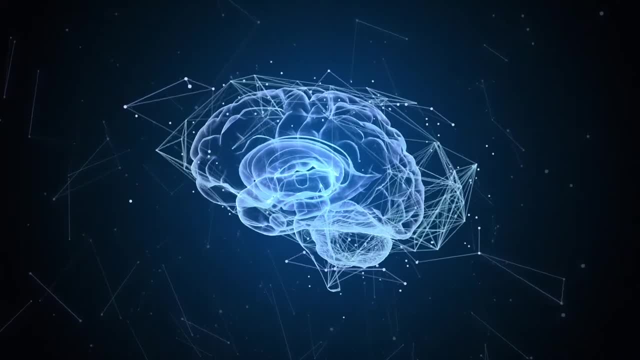 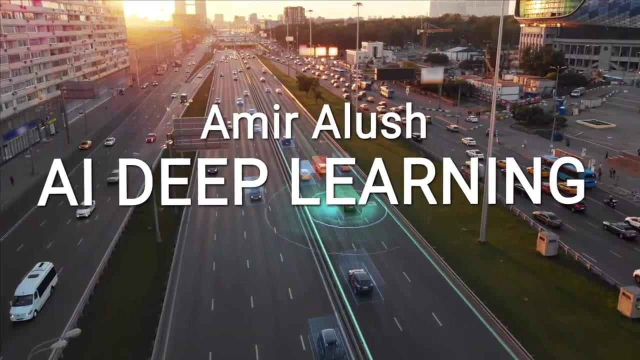 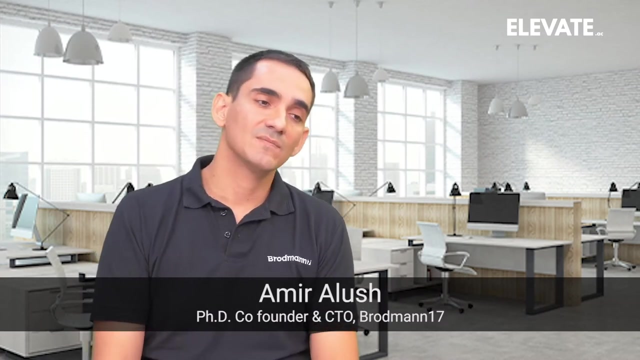 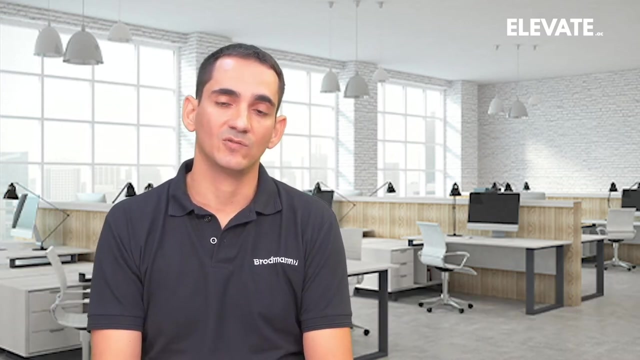 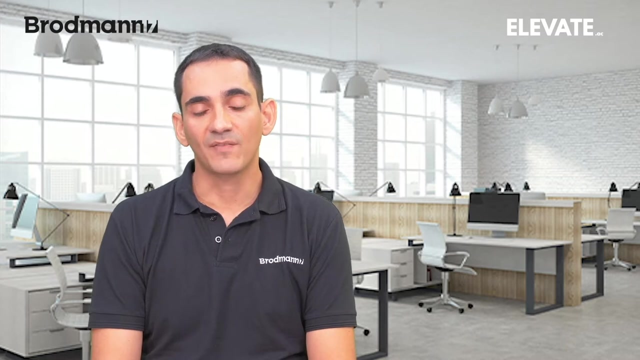 So I would say that, in terms of adoption, so we see this large movement towards, towards adding this AI and making our vehicles safer. So I think the current expectation that within a decade you would have these capabilities, these AI capabilities, within around 120 million vehicles around the world, In my opinion, the main inhibitors for this- 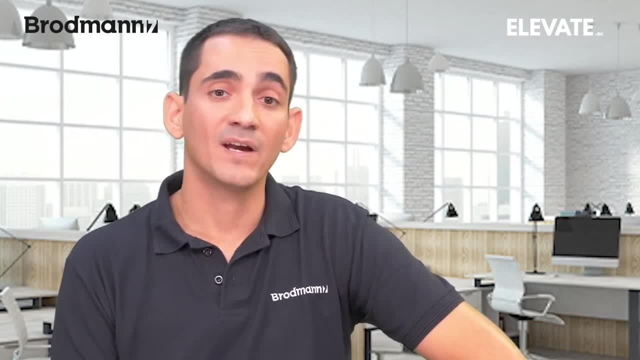 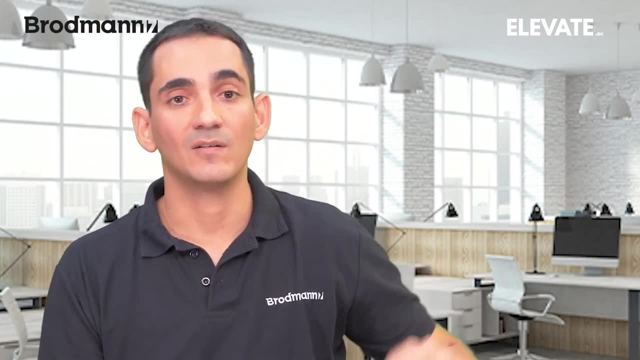 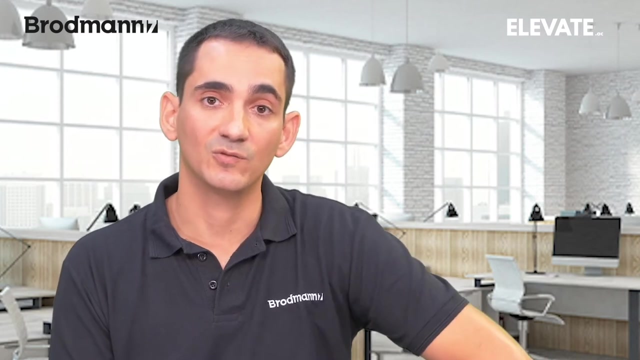 massive scale up of AI are two. One is accuracy. We'll have to basically close the gap between the level of accuracy we get today in level one and two and the level of accuracy we need to get in level three, level four and especially level five. There is a gap to close. there. Many companies are working on closing this gap. Perhaps you've heard on Waymo. So far they've driven around 20 million miles in public roads and did in-lab simulation of around 15 billion miles. All of that in order to assess the level of accuracy needed. 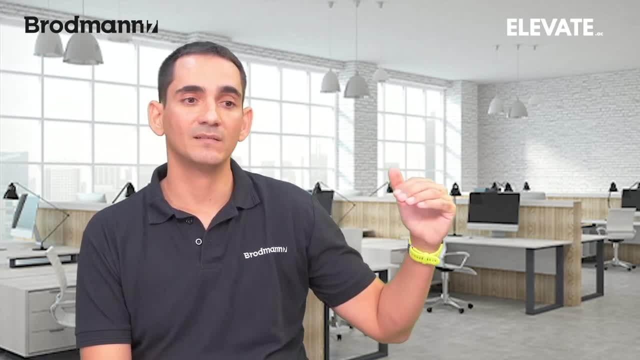 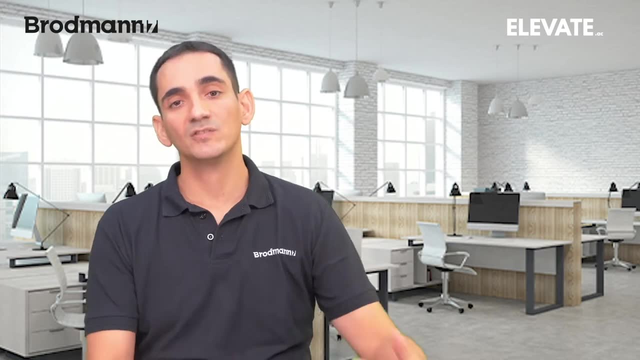 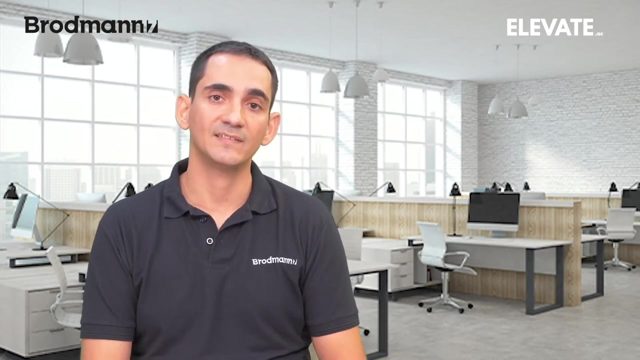 In terms of level one, level two, I think we're in a quite a good place. Statistically, the machine learning algorithms or deep learning algorithms inside level one and level two do not currently reach 100% accuracy, but statistically they do cover all required functionality. 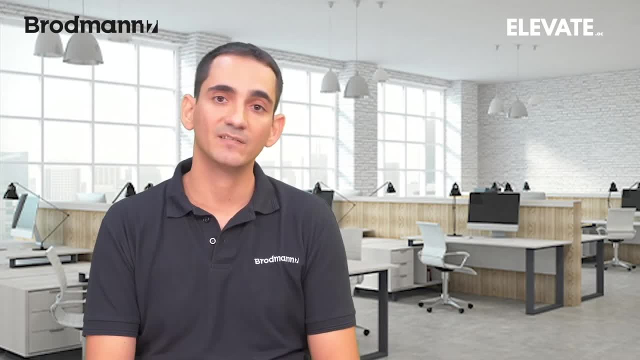 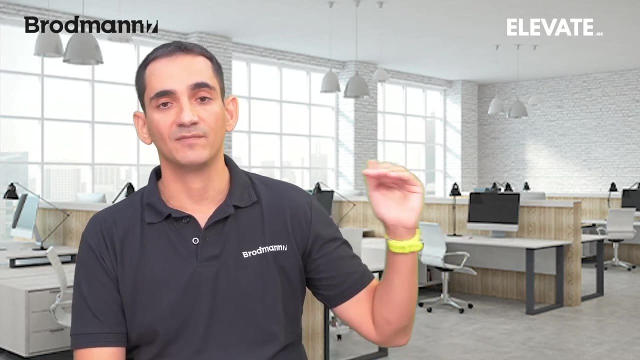 especially if we're talking about the limited scenarios you expect them to engage in, right When you're talking about level three, level four, level five, the broad amount of scenarios, the complexity, this level of accuracy level one and level two have today. 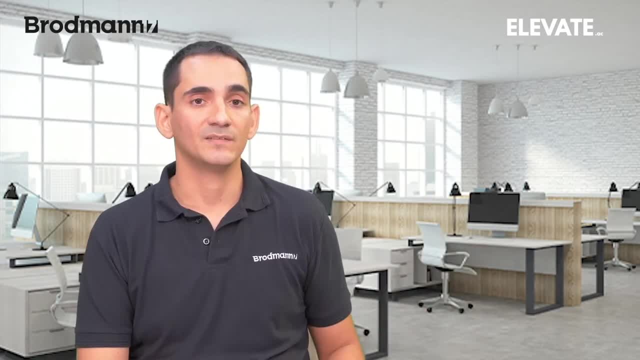 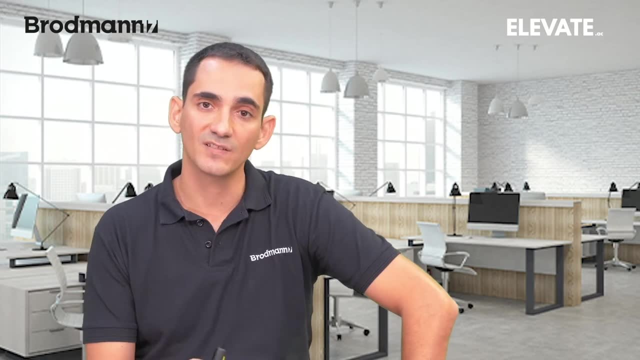 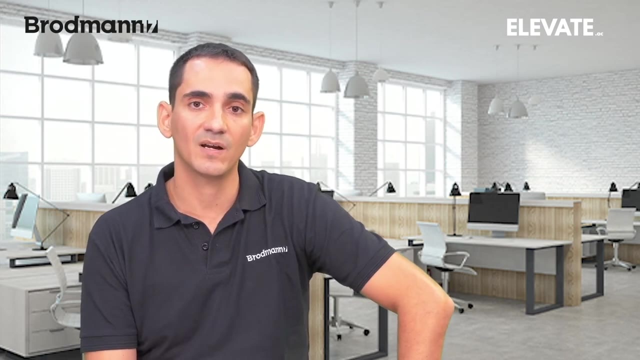 is not enough, So we need to close this gap. There is a lot of effort being put into developing stronger processors, So compute is also another issue we need to overcome. Today, when you're talking about premium vehicles, if you look at Tesla, for instance, they have their full 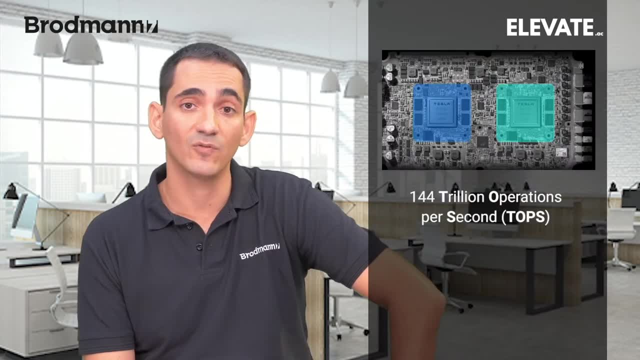 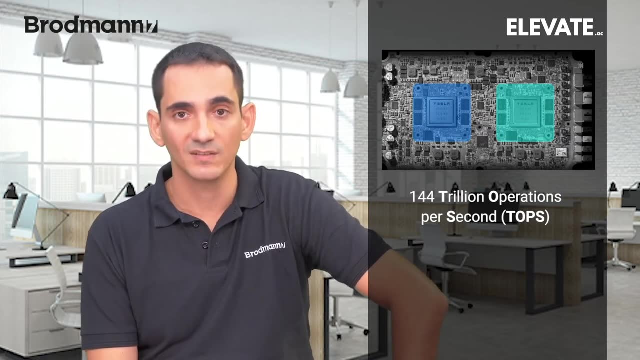 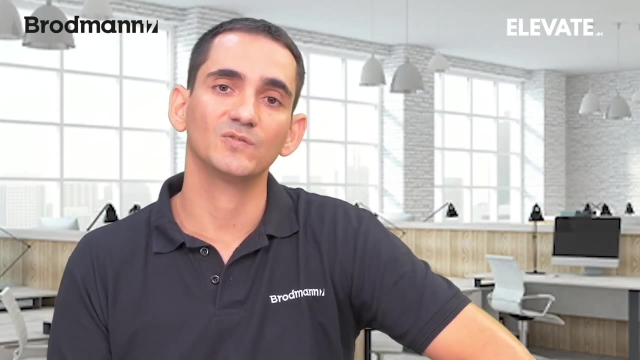 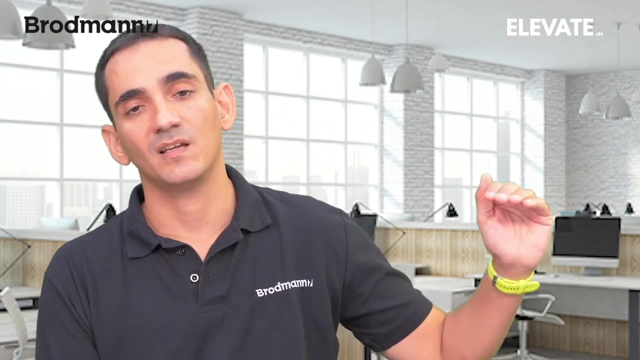 safe driving computer. It has around 144 TOPs of compute power. TOPs is basically an indicator of the amount of compute the hardware can do. So they've actually developed this custom-made hardware in order to support the full capabilities they believe will be sufficient to support a fully autonomous.